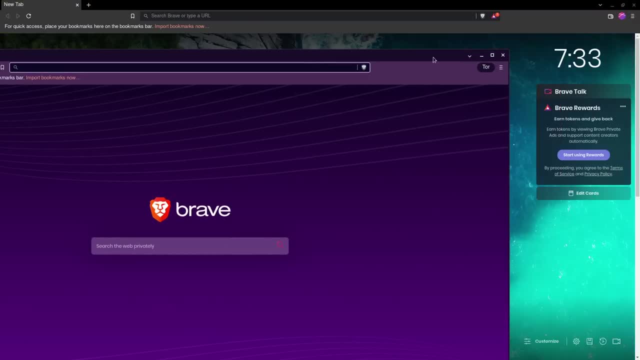 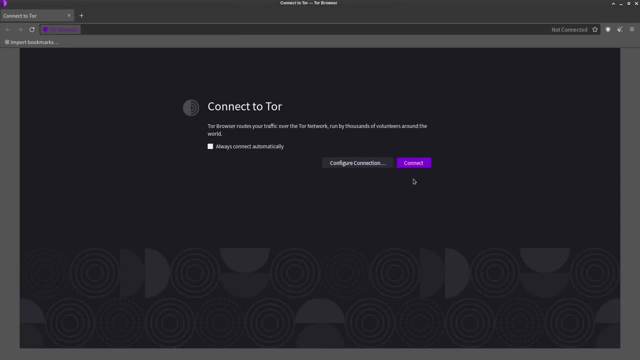 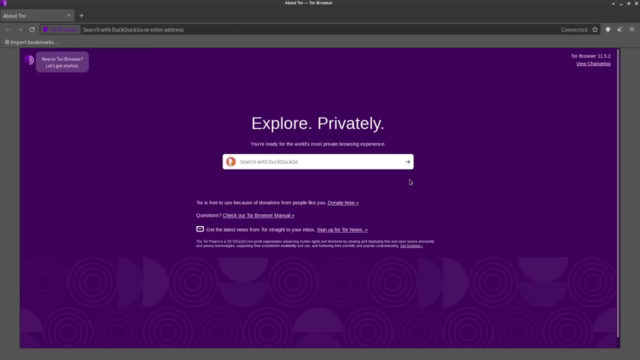 you know it's not recommended to do this, but it is technically possible. But anyway, let's go to what is recommended. So when you first open up Tor, it's gonna look something like this and you just click connect And bam, now you are connected to Tor using the Tor browser bundle- So easy. 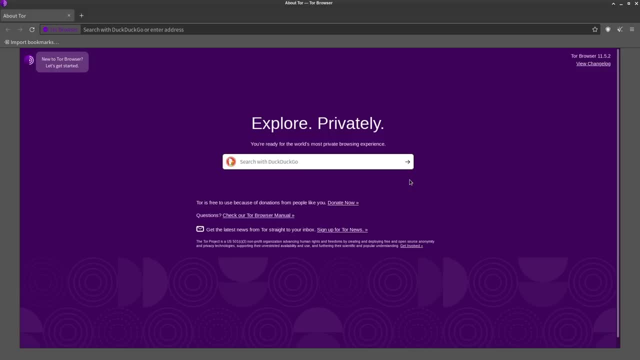 parts out of the way. but how do we really get to the dark web? Well, really, the dark web is just websites and services that end with onion instead of com or org, and you can only access them using special browsers like Brave, when connected to Tor or the actual Tor browser. But the really tricky 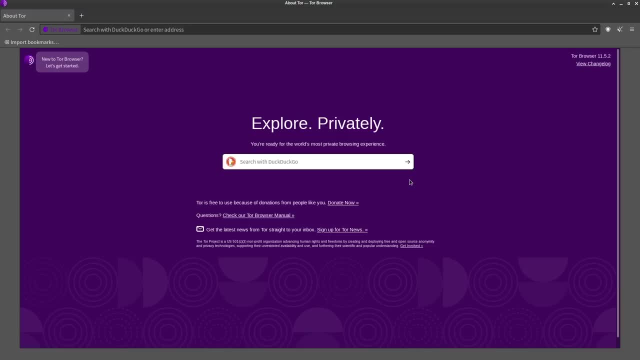 thing about these onion sites is that they're all made up of 54 random alphanumeric characters, So you're not going to be typing those in like regular websites. you know, like youtubecom, You're not gonna be able to remember onion site addresses, So you need a direct link and that is where sites like 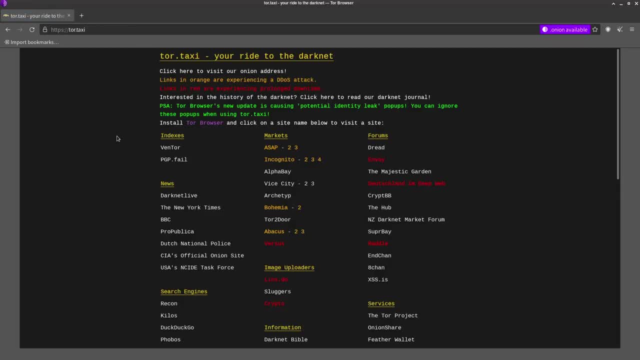 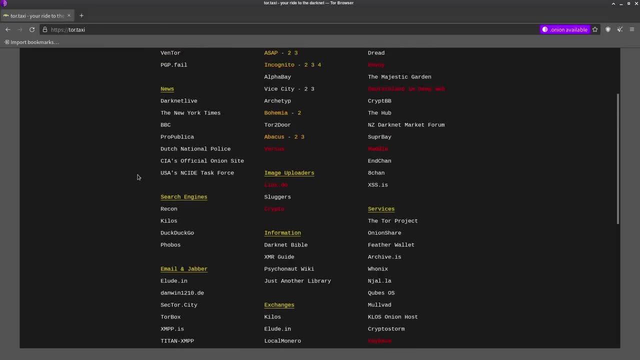 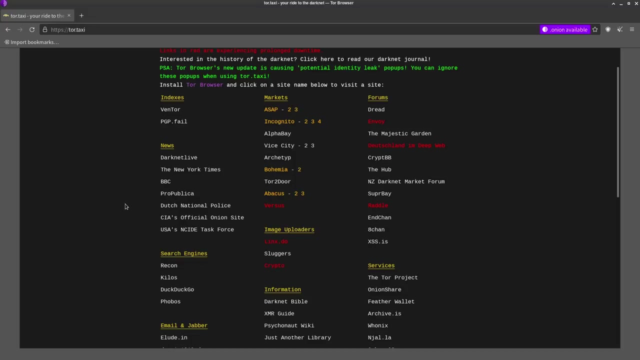 tortaxi come into play. So here you can find links to various dark web sites, categorized by types, and you can also have some confidence that these links are going to go to legit sites and not scams, at least as long as you're using. 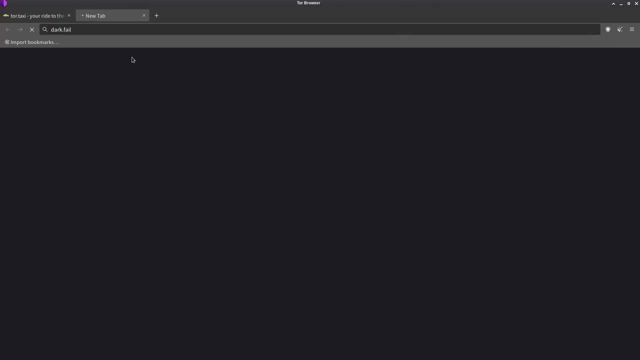 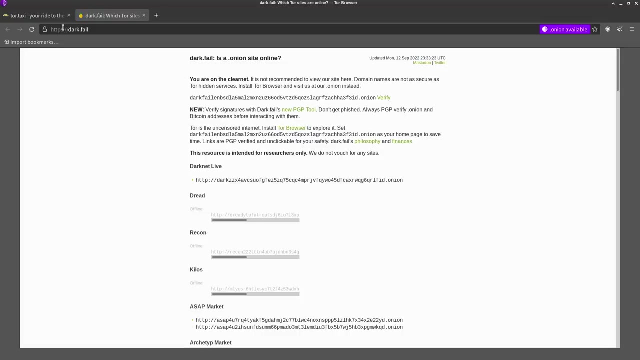 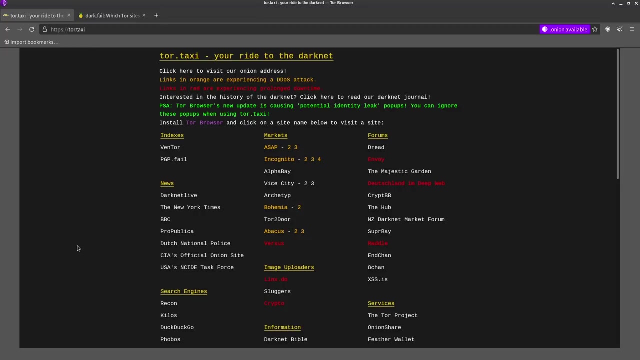 like tortaxi or darkfail is another really popular one, where they're reputable, they link to legit sites, so on and so forth. I guess also as long as they don't get hacked right, because then somebody could change them. But anyway, if I mouse over these, you see all these different onion links that are 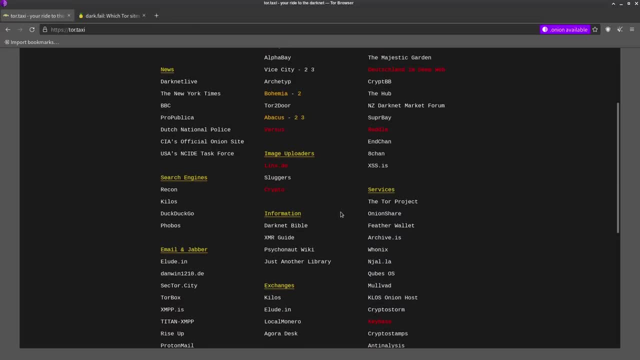 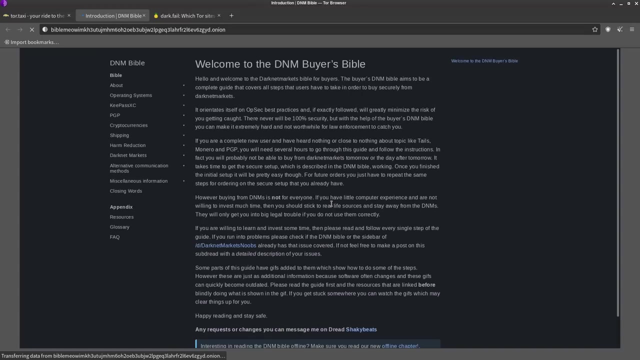 in the bottom left hand corner, And some things that you might want to take a look at here, especially if you're new to Tor, is things like the Darknet Bible. So what this covers is OPSEC, and it has it broken down into different subjects like 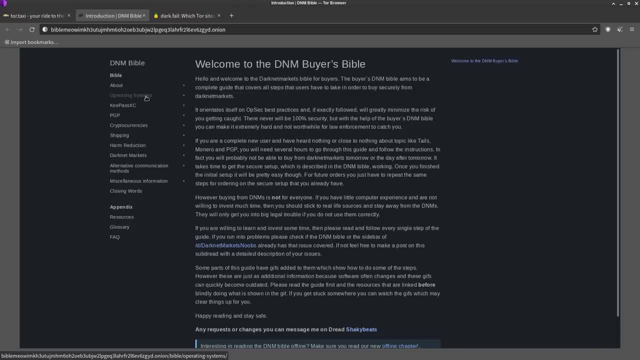 operating system. You know they're gonna tell you: hey, you don't use Windows and probably use like tails or Hoonix or cubes, things like that. You know KeePassXC. Even if you're not using Tor, you should be using KeePassXC Everyone. 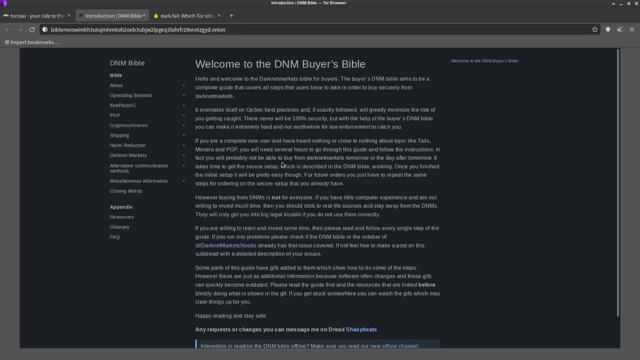 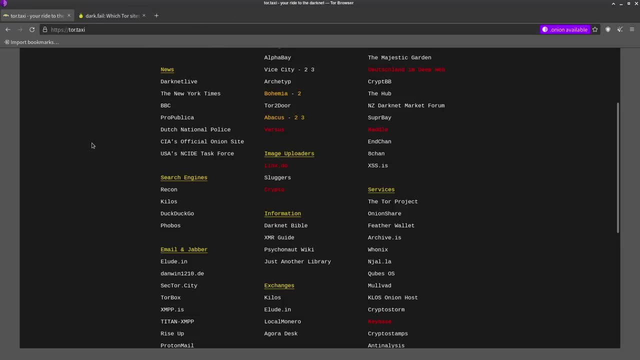 should be using a password manager, PGP and so on, But this goes a little bit beyond the scope of this tutorial. right, We just want to kind of explore the dark web. Oh, and one other thing that I just want to mention while I'm thinking about. 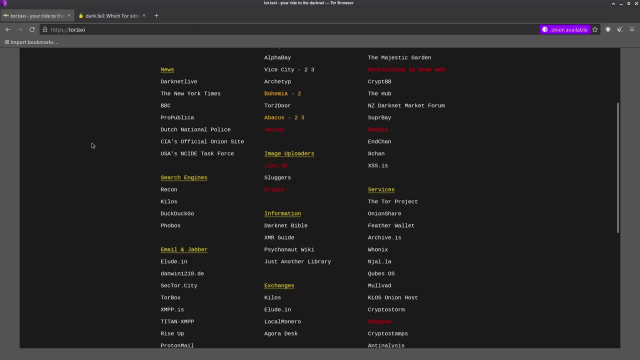 OPSEC is. I see so many beginners asking this- if they need a VPN or whether it's good to use a VPN with Tor. Like, I guess people connect to a VPN and then they go and connect to Tor And the answer is no, Okay when you're using Tor. you're already getting way better anonymity than any VPN could possibly provide you. The only possible benefit that you might get with using a VPN with Tor is that if you live in a country that blocks Tor Or you're using an internet connection where the network administrator is, 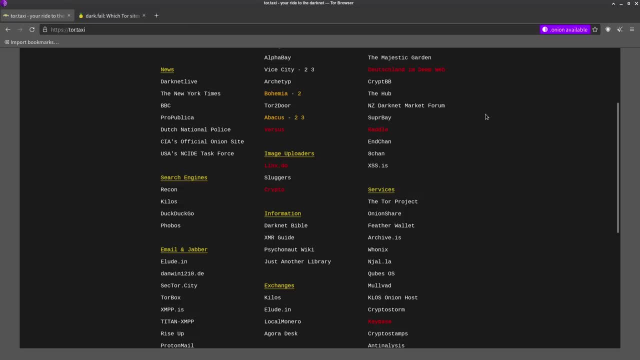 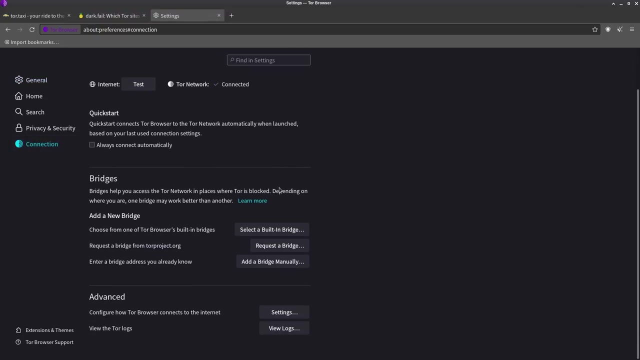 blocking Tor, Then using a VPN, would be able to go around that. However, there's already options to get around the censorship built in toward So if we go into their hamburger menu, And I think it's in settings and connections. So bridges, okay, bridges already. 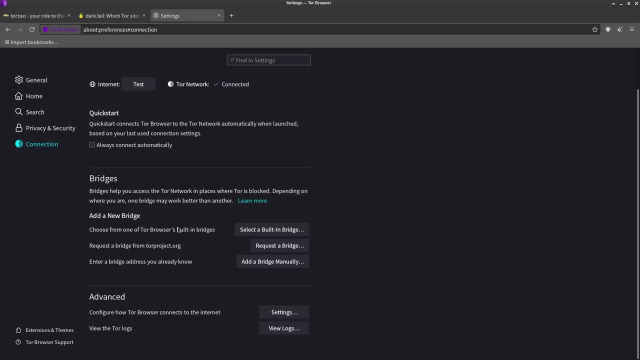 accomplish that for you. So if you're in a country that's censored Tor, you're using a network that centers Tor. Try using this to get around it. No reason to use a VPN with Tor. That's just. I have no idea who is responsible for starting that silly trend, but I just. I see it. 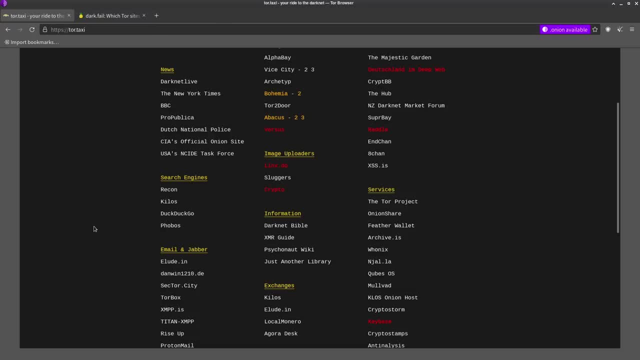 all the time when people are talking about Tor: Oh, do I need a VPN? No, you don't. So let's start looking at some search engines to actually find some stuff. Now, the only real dark web search engine in here is Phobos DuckDuckGo. that's a clear web search engine. you guys are probably 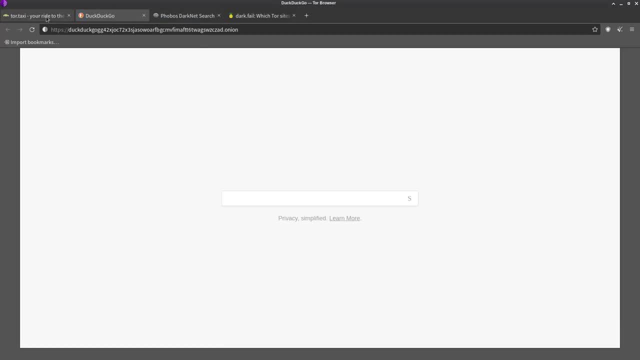 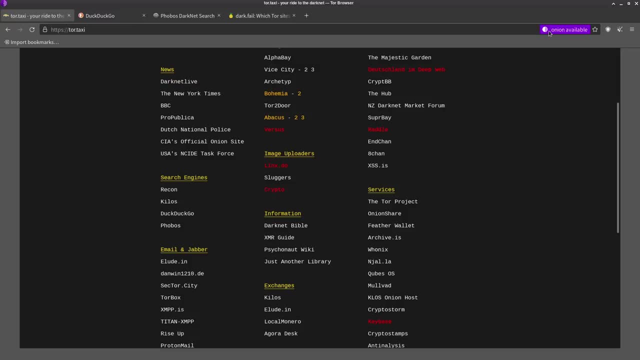 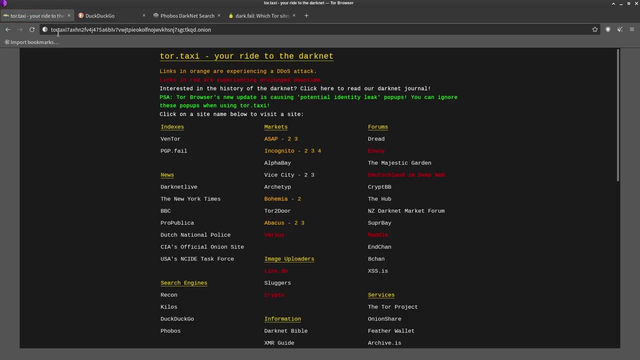 familiar with, but this is just their onion domain And, by the way, lots of sites on the clear web also have onion domains available. You'll be able to see that in the upper right-hand corner. So, like TorTaxi here, if I click on that purple onion domain available, it changes to the onion link. 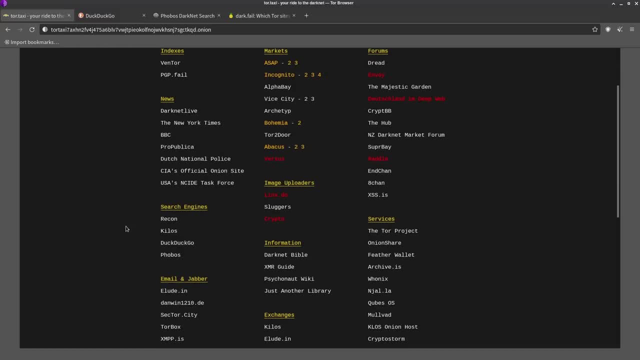 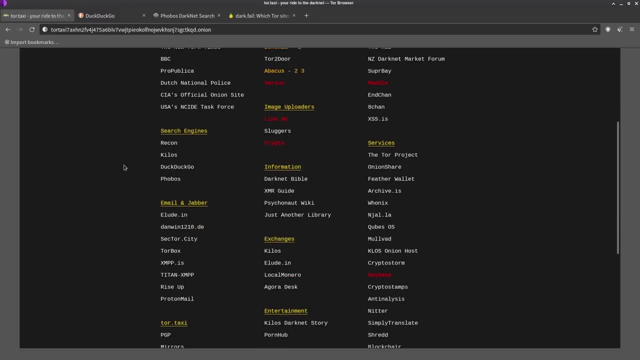 and now we have a little bit better information. Anonymity, because now we're not having to go to an exit node to get to this website, which I don't really like exit nodes because personally I think a lot of them are operated by law enforcement. 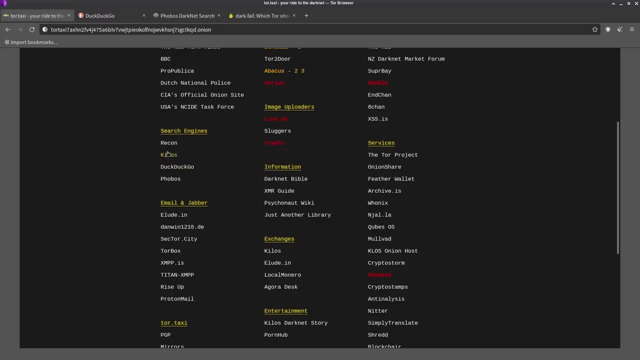 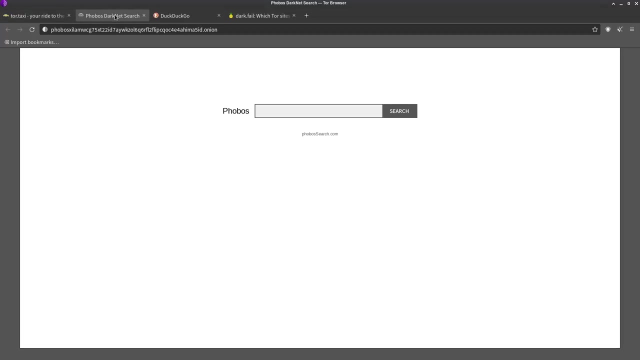 but that's again beyond the scope of this video. Recon and Kilos: these are also different than regular search engines. These are more for like searching dark web marketplaces specifically. right, But if you just want to dig into general things, Phobos is a good. 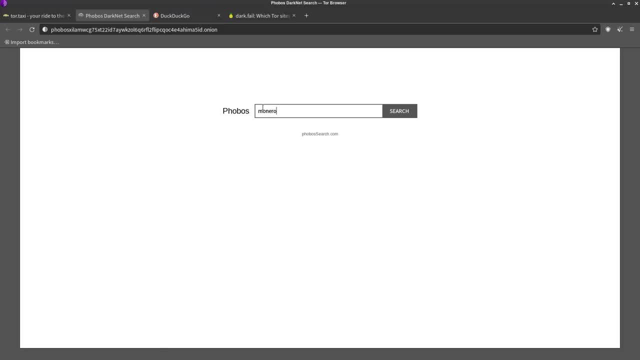 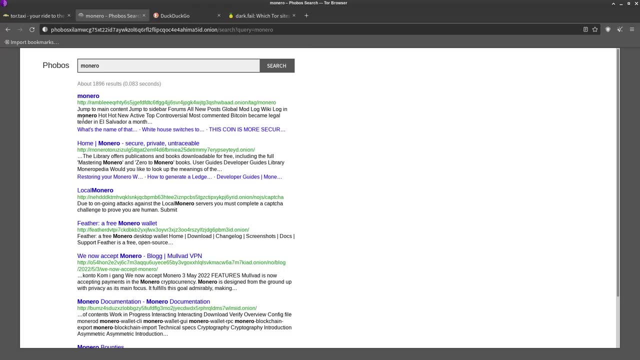 good place to start, So we can look up something like Monero, for example- right, Pretty popular subject on the dark web, also a pretty cool cryptocurrency, And you can see all of these results that we're getting. these all go to onion domains, And so this is how you start going down. 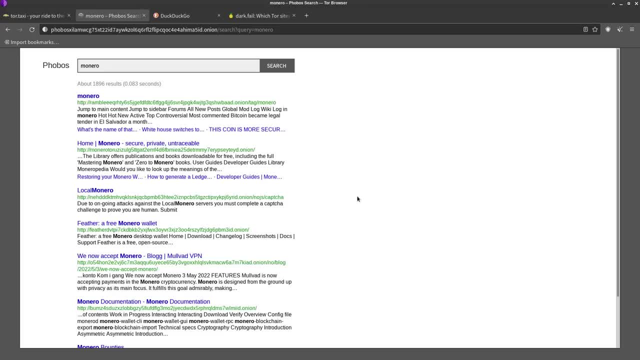 the rabbit hole of the dark web. right You start going to these different onion sites and these are probably going to link to more onion sites. You know what it's like. actually, Zoomers won't get this, but the older people. 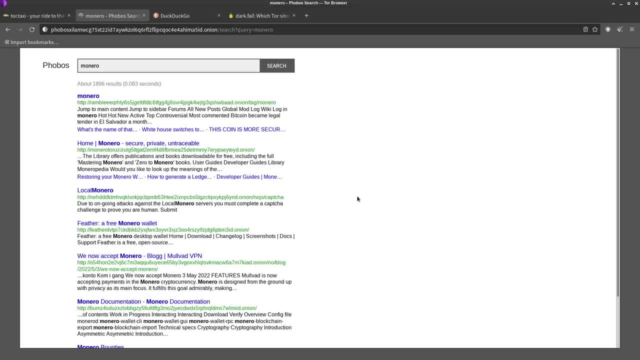 browsing the dark web is a lot like browsing the internet before they had search engines. right Now you can just bring up Google or you know whatever search engine and find a whole bunch of stuff. But way back in the early days of the internet you would have to go to one site. 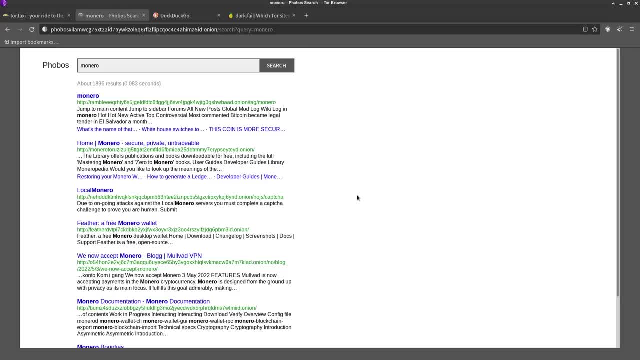 and then that would link to some other sites, and that would link to other sites, and so on and so forth. Now, Phobos is not the only search engine that's out there. right, You want to find more dark web search engines? We can just type in, you know, search engine, search engine, search engine. 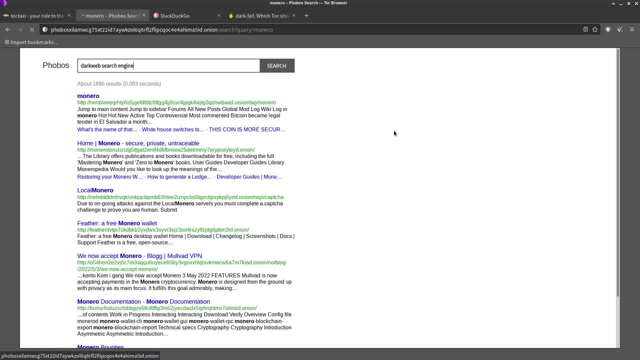 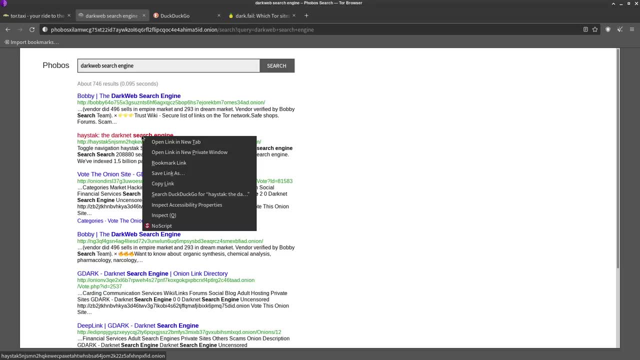 type in dark web search engine And ho, look at that. We got a whole bunch of results. We got Bobby, which I don't actually know, the search engine, so I'm not going to click on it. It might be a little. 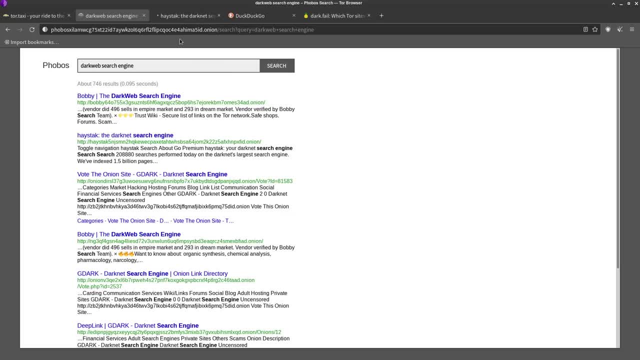 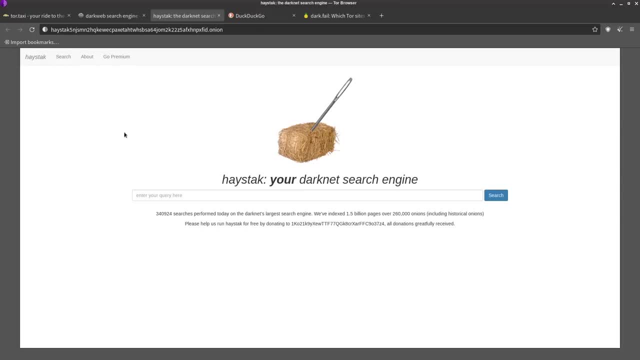 bit sus. Haystack, I think, doesn't have any crazy ads on the front page. Actually, let me just drag this over here and check. Okay, Yeah, Haystack looks safe. Another little quick tangent. So a lot of sites, especially search engines. they don't have any crazy ads on the front page, So 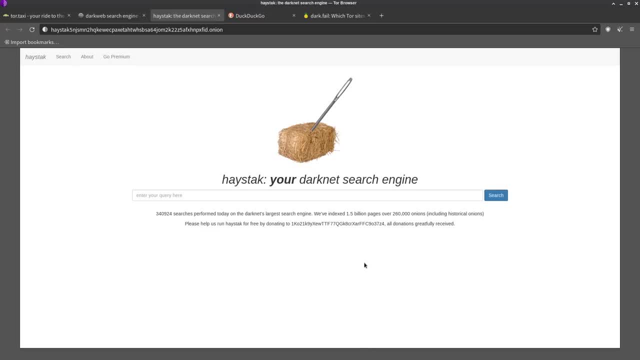 search engines on the dark web, they'll have a whole bunch of ads that load for various services on the dark web And you know, given the nature of the dark web, a lot of these services are illegal. So if you're using the dark web in company or you know somewhere where I don't, 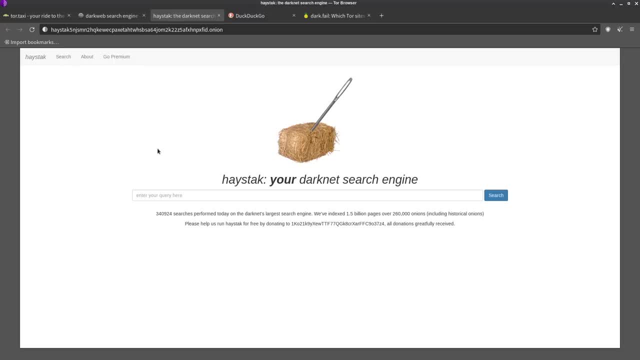 know, maybe you're in public and like a camera might be looking at your computer screen. just watch what sites you're going to. right, If someone sees you looking at illegal stuff on your computer, they might try to- I don't know- call the feds on you. So yeah, this is another dark web. 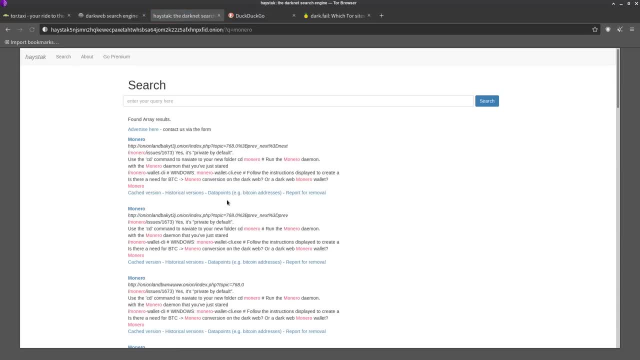 search engine. We can go ahead and type in Monero, like we did, and then we're probably going to get links to other places. because all of these search engines, they're not always going to have the same indexes. Sometimes they will. I guess it depends on what indexes they use, but obviously 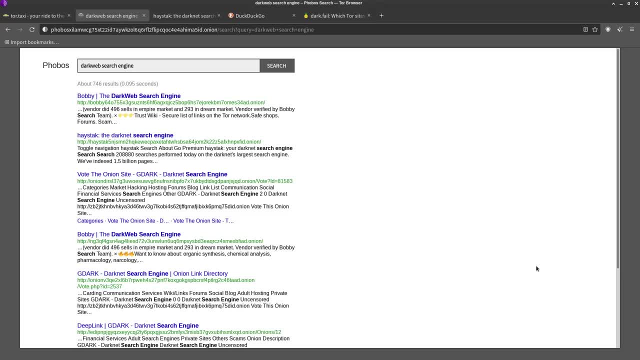 Haystack and Phobos are a little bit different. Okay, So, now that you've found some stuff, how do you save this right? Because chances are, if you're just starting to explore tour, especially if you didn't know about tour taxi and Haystack and Phobos and all these things. 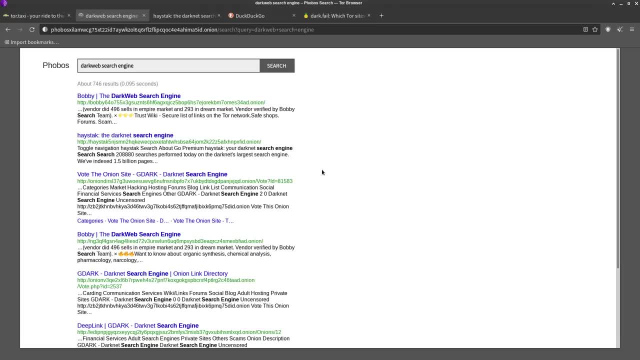 you're probably going to be going on a you know days, maybe even weeks long expedition looking up all kinds of different stuff. I mean, I remember back when I was in high school and I first learned about tour. that was like what I did for probably a month, maybe two months. 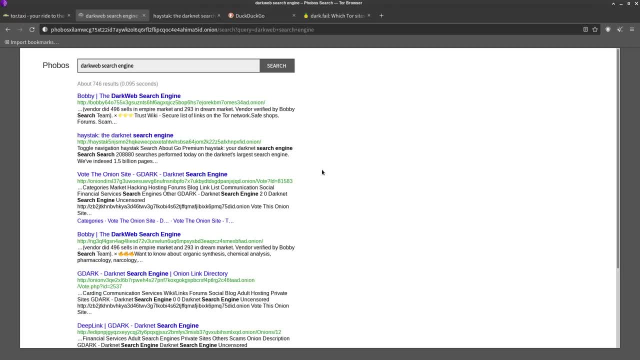 like no video games, like no nothing else. I just wanted to explore The dark web. It was cool, Um. so how can you uh sort of keep tabs of what type of sites you've been exploring? Well, one thing you could do is you could just bookmark them. 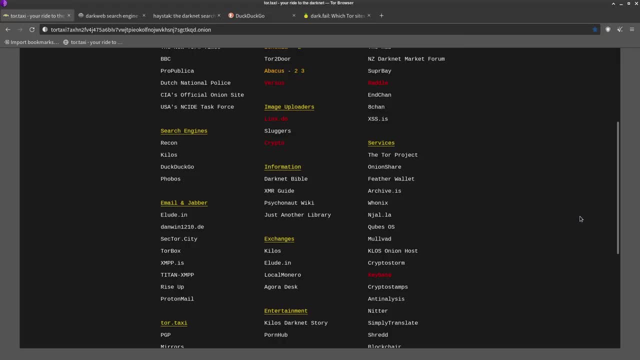 in the uh tour browser, right, I mean it supports bookmarks like pretty much any other browser. but this might not be a very good idea, depending on what kind of sites you're going to right. Tour taxi: Eh, maybe it's not that bad to bookmark tour taxi. I mean it does have. 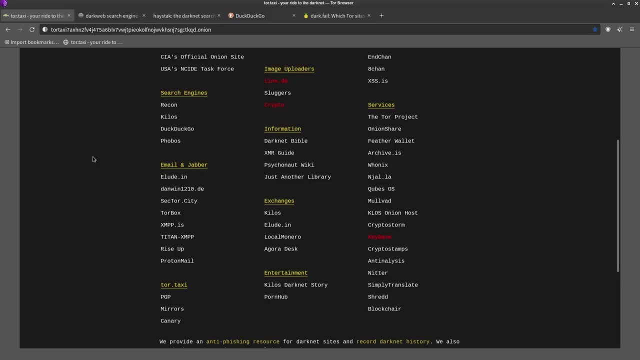 links to. so you know that might be a little bit sus, but it's not necessarily illegal links to markets, at least not here in the U? S. your country might be different, Um. so you know, having these bookmarks in the browser might be a bad idea, because if your computer gets seized or somebody else, 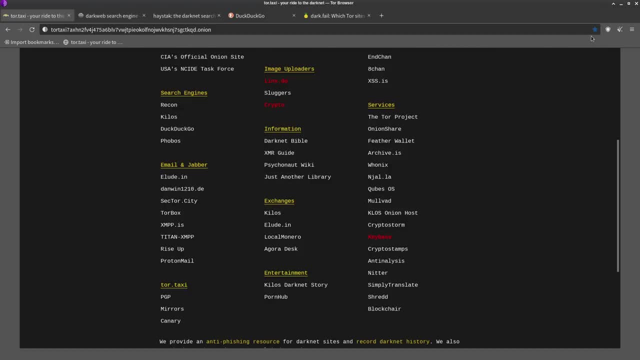 you know, uses it and opens up tour. they're going to see all your bookmarks, They're going to see what you're going to. So that might be a bad idea. What is a better solution? Well, um, one thing we could do is we could just.